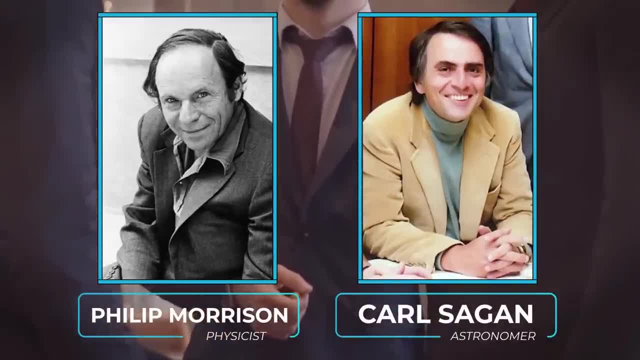 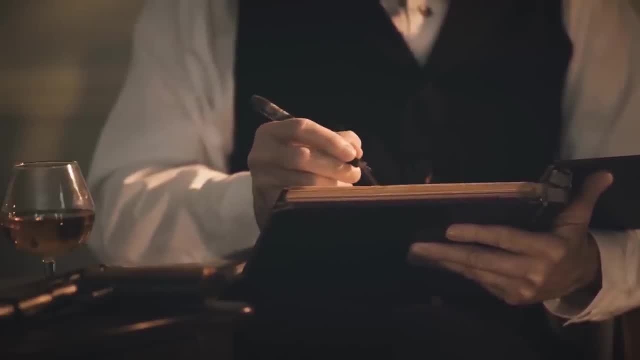 Carl Sagan was both in attendance. Drake said that he came up with the equation a few days before the meeting, largely as a way to come up with an agenda. Each term in his equation was meant to serve as a discussion point for the attendees. 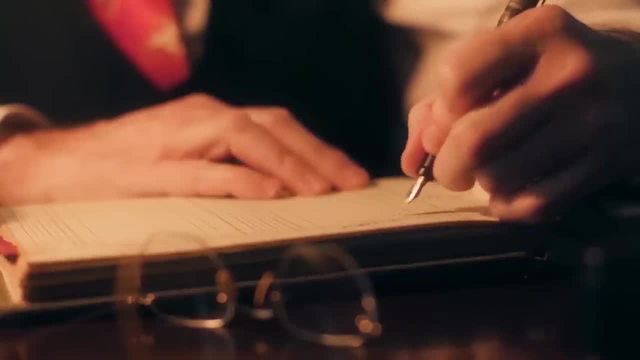 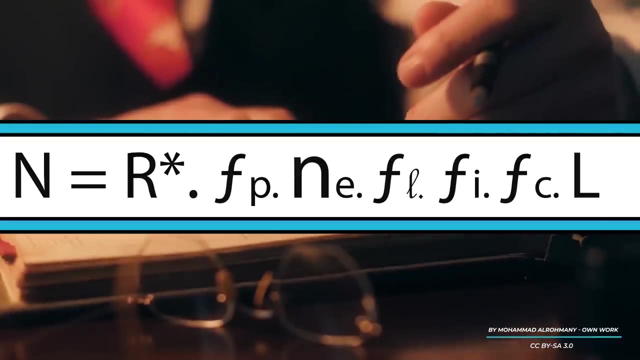 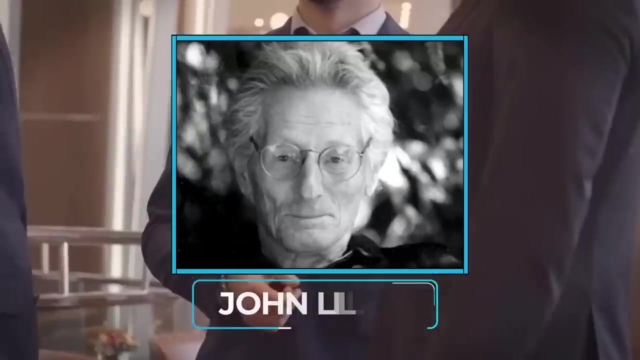 Now we don't know precisely the form that Drake wrote down at the meeting, but the canonical formalism was first published by Drake in 1965.. After the original meeting, the participants dubbed themselves the Order of the Dolphin, inspired by attendee John Lilly's. 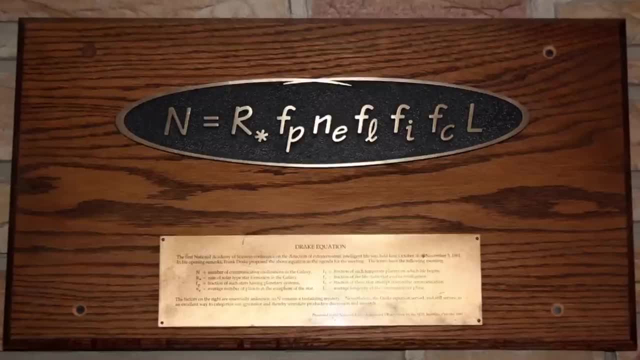 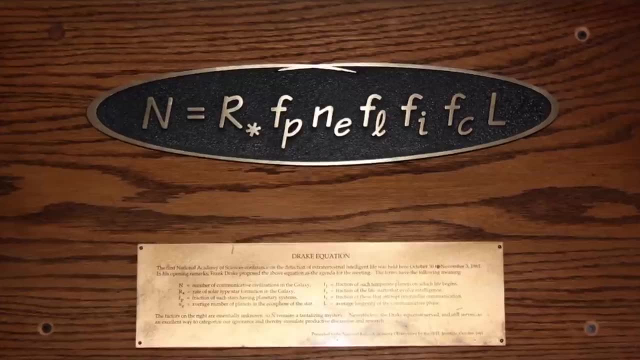 research on dolphin communication. The meeting and equation were even commemorated at Green Bank with their plaque, which is still there and worth checking out if you like astrotourism. Clearly, then, there was a sense that this was a rather historic meeting. 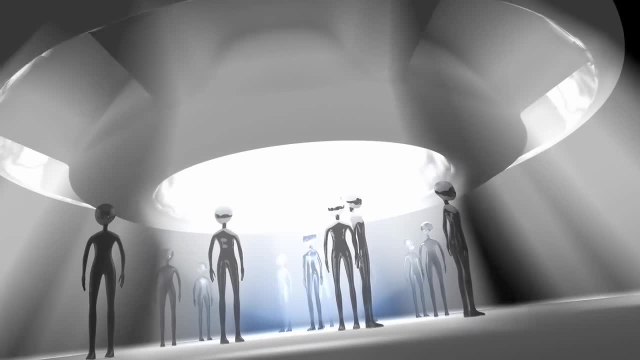 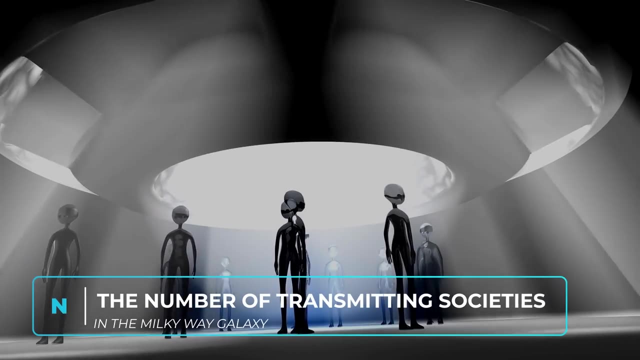 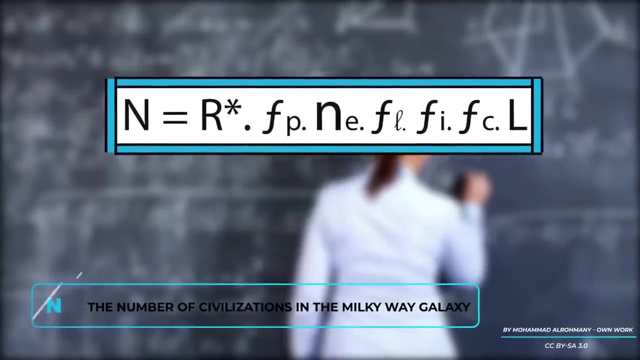 But what exactly is the Drake equation? The Drake equation estimates N, the number of transmitting societies in the Milky Way galaxy. Let's take a look at it. The terms are defined as follows: N equals the number of civilizations in the Milky Way galaxy whose electromagnetic 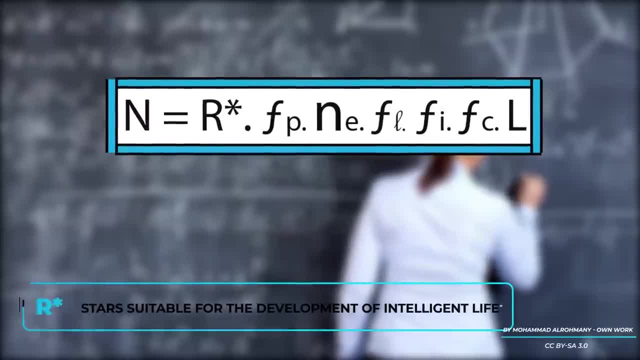 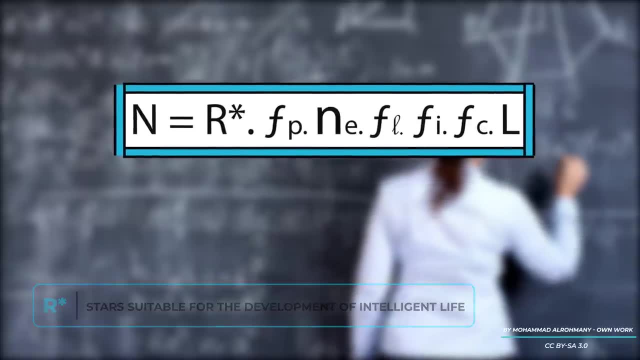 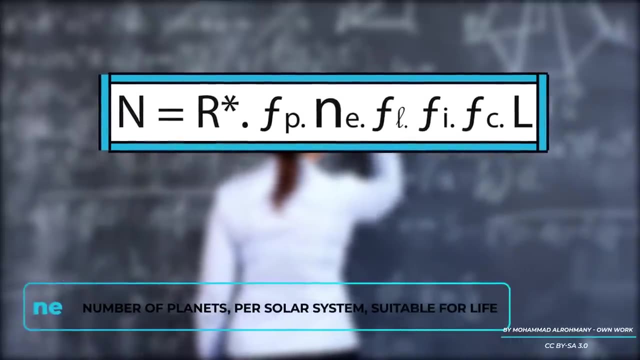 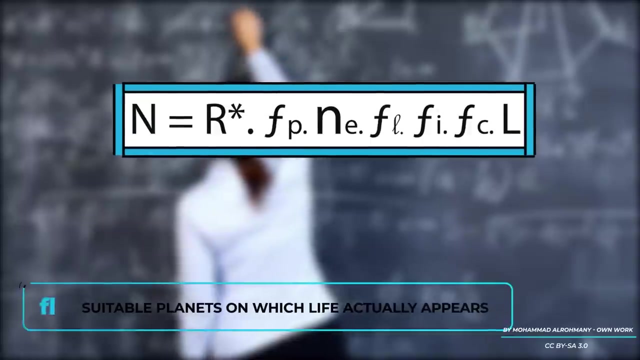 emissions are detectable. R equals the rate of formation of stars suitable for the development of intelligent life. The correction of those stars with planetary systems. The number of planets per Solar System with an ambient suitable for life. The fraction of suitable planets on which life actually appears. 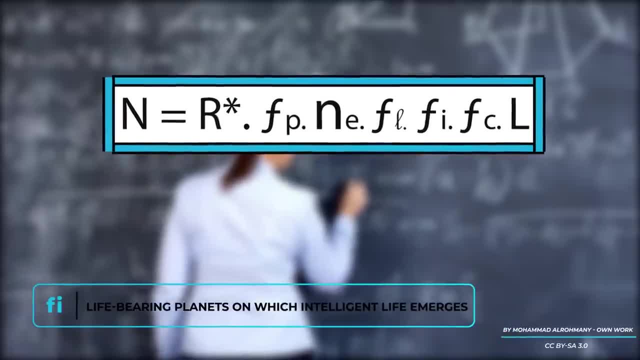 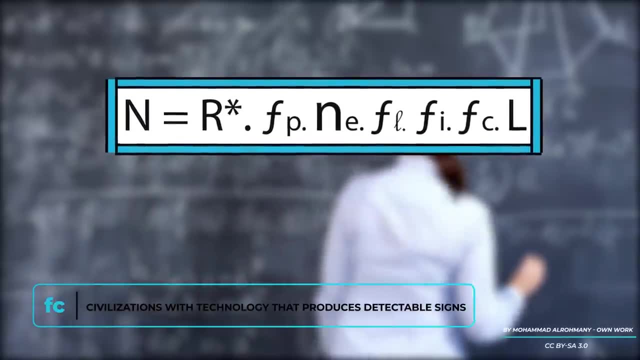 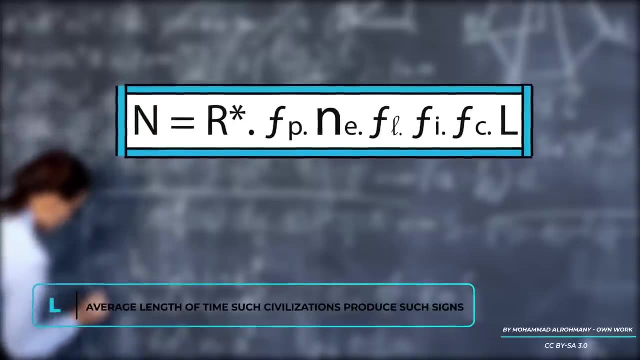 Xiaomi equals the fraction of life-bearing planets on Sagittarius which intelligent life emerges. Fc equals the fraction of civilizations that develop a technology that produces detectable signs of their existence. L equals the average length of time such civilizations produce such signs in years. 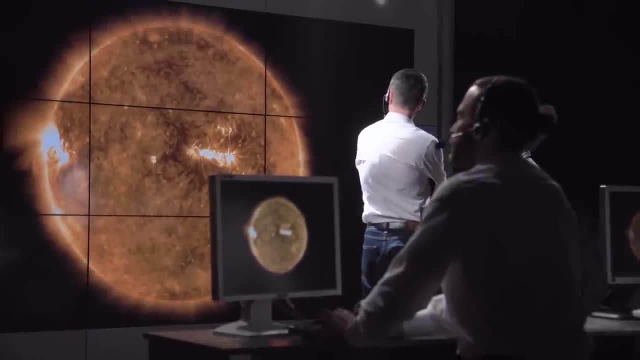 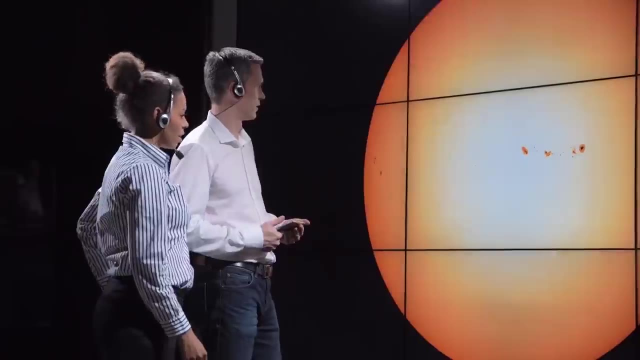 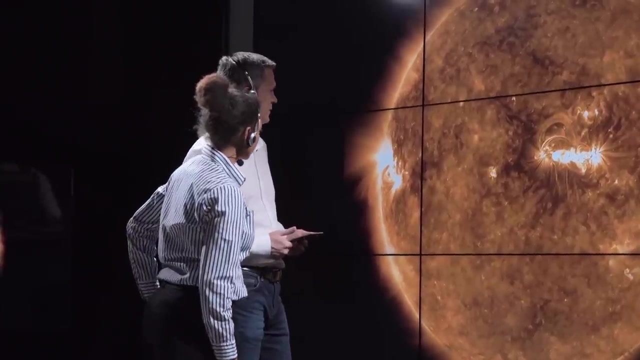 Currently, there are 100 scientists at the SETI Institute working on nearly 100 research questions, But each of these topics can be related to one of the terms in the Drake equation. Looking closer, the anatomy of the Drake equation can be grouped into just three types of variables. 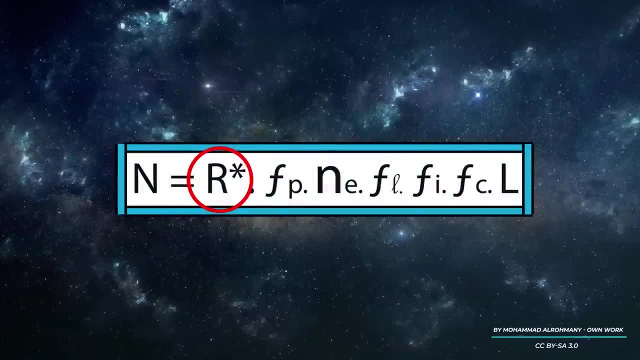 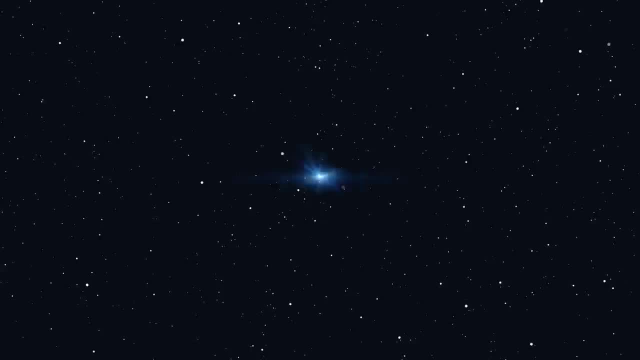 We have a rate as the first term that has units of inverse time. For example, the rate of stars is x per century or y per year. It tells us how many stars are forming in the Milky Way in a year or in a century. 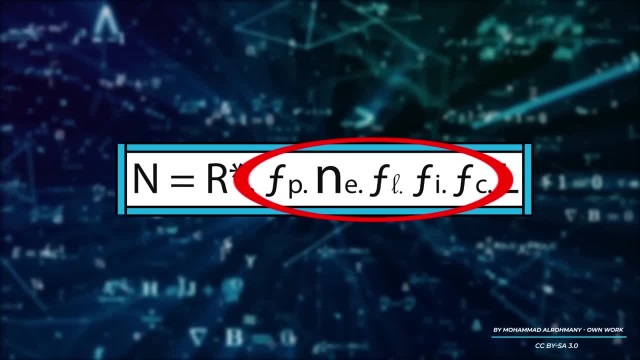 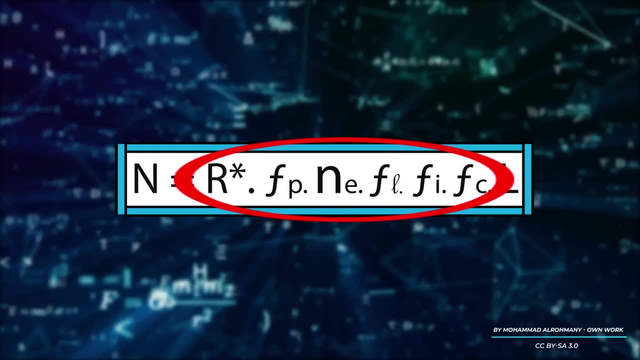 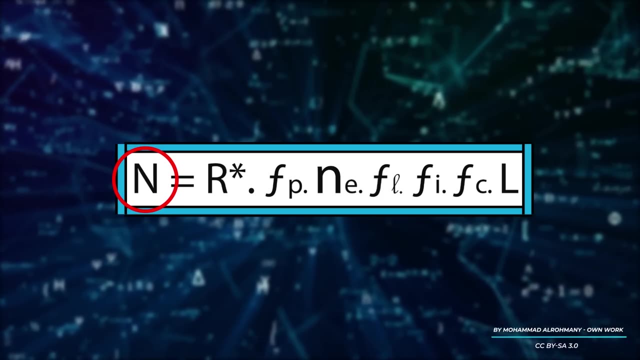 Next we have a bunch of fractions and numbers and quantities without any units. Okay, since we have a rate multiplied by a bunch of numbers, then the first six terms must all represent a rate when combined. But the Drake equation calculates n, and n isn't a rate. 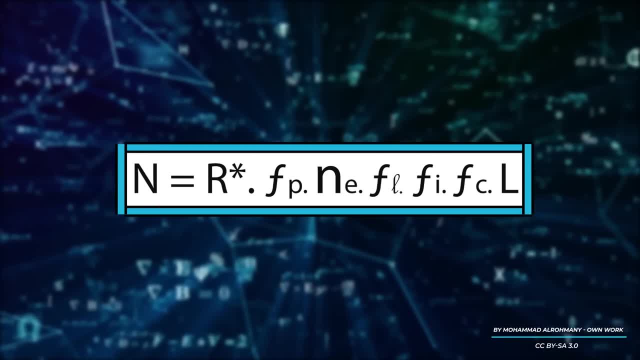 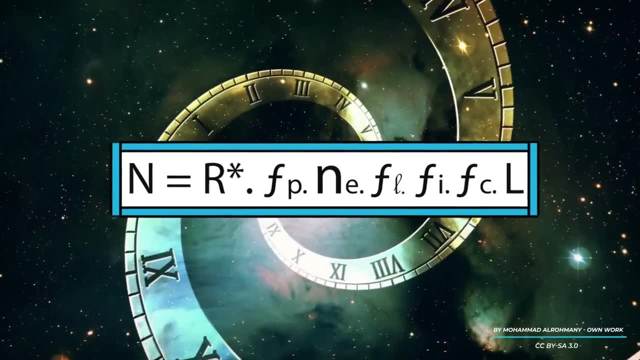 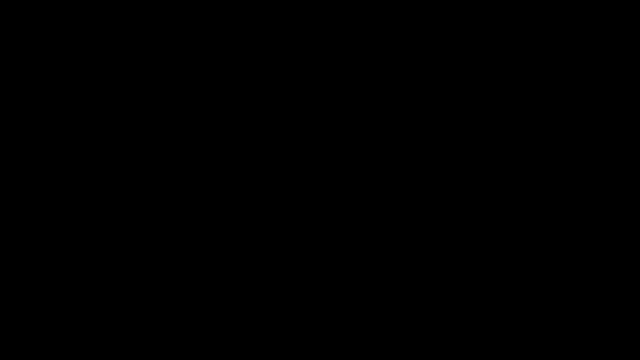 To get rid of the rate, we have to multiply by a time which, in this case, is L, the mean lifetime of civilizations. That's all Simple, Elegant, The Drake equation. But can we say something more? Of course we can. 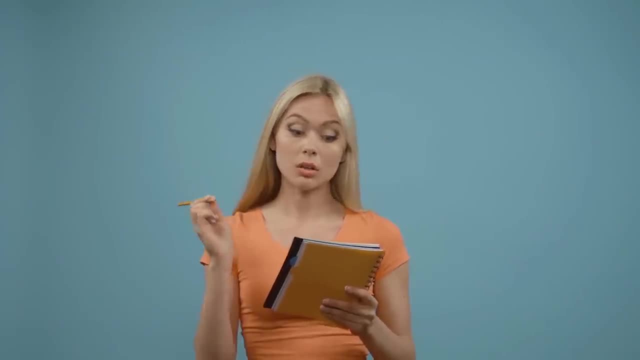 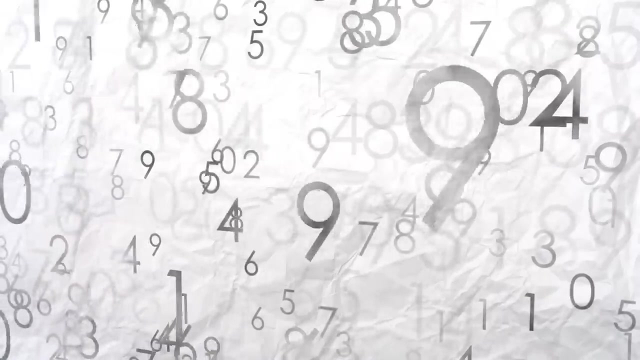 Can you see what's the problem with the equation? I bet you see it. The problem is: what are the parameter's values? Of course, we can go ahead and plug in guesses for these values, and that's actually what the original attendees did. 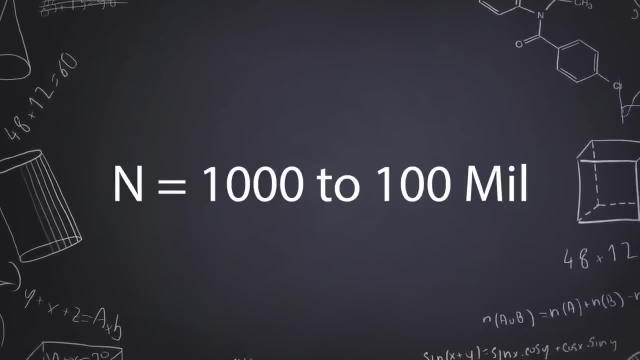 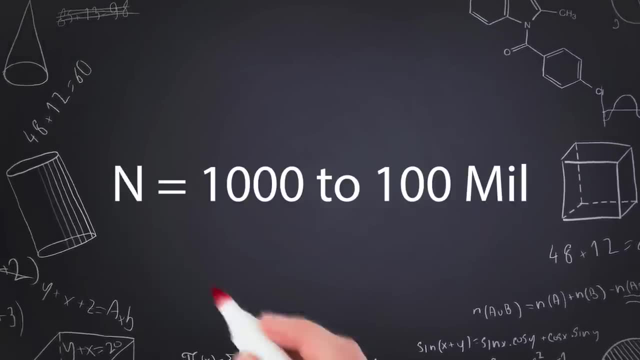 Arriving at a final estimate of n between 1,000 and 100.. That's a total of 300 million. But let me emphasize in the clearest possible terms: Those are just guesses. J, Our problem is that it's not possible to evaluate the formula. 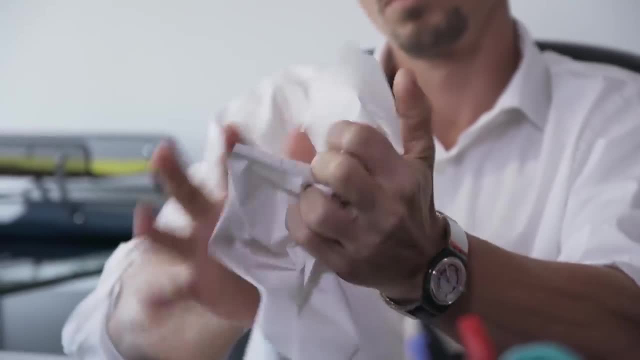 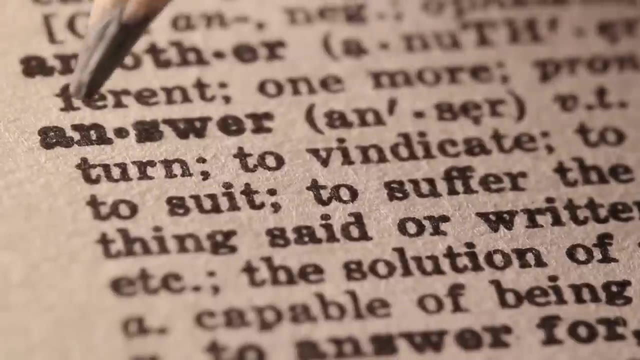 in a conventional sense, because we simply don't know the values of most of these terms. Humans are ignorant. We have to deal with that. As we said, we don't have all the answers, We have just a few of them. In the case of the Drake equation, we have only one. 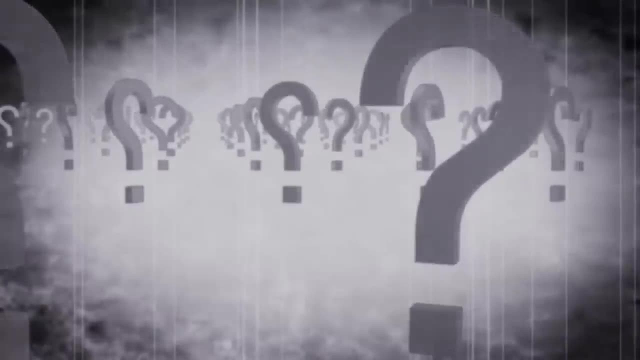 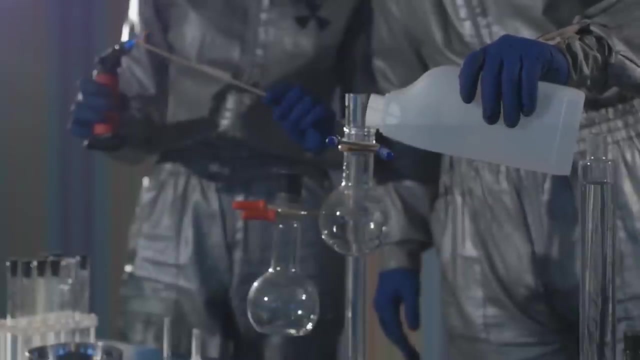 We have two. This is the answer. We have only one. We don't know the values of the terms And anyone can guess, And your guess is as good as mine. Even a child can use it- And here we have a recipe for disaster. 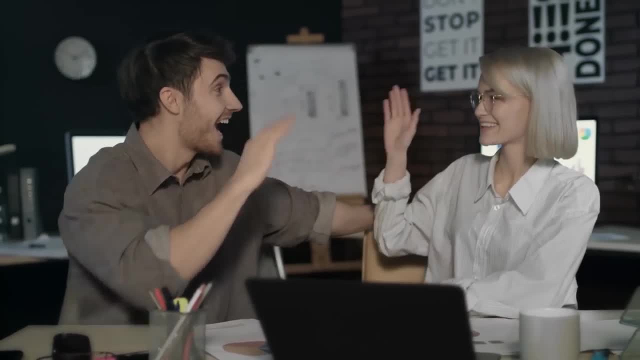 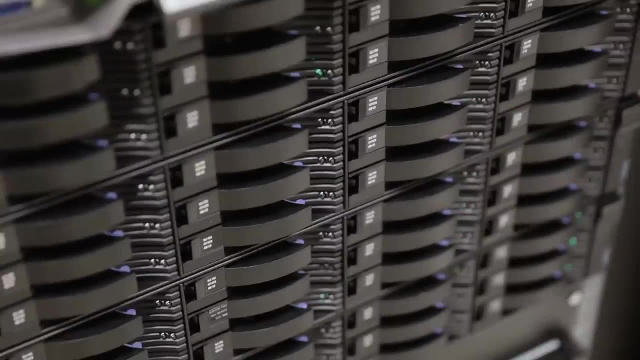 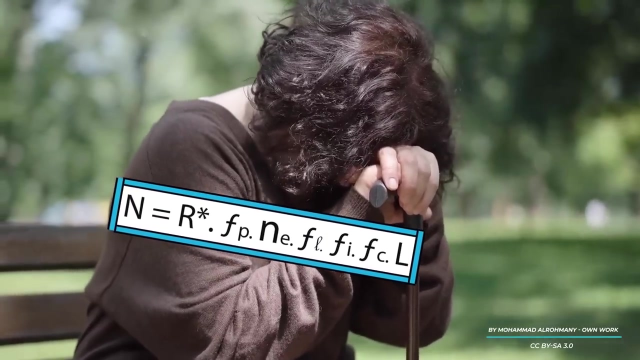 We end up with a situation where lots of people can come up with their answers and claim them. as a result, There have been enough previous studies on this topic to fill a small hoard of hard drives. in many ways, The Drake equation is a victim of its own success. 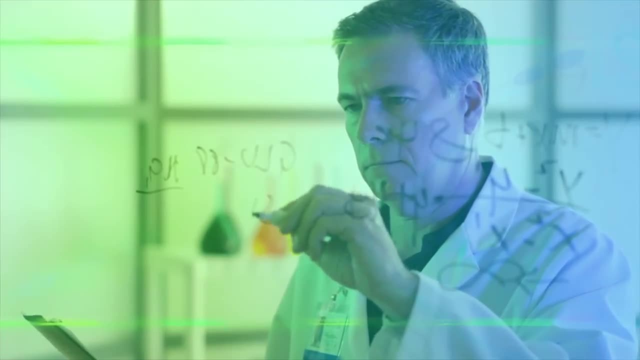 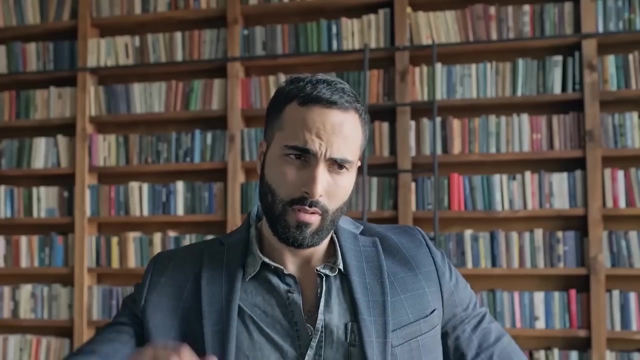 It seems that every month or so, we hear about a new study that plugs numbers into the equation and arrives at a different answer. None of this teaches us anything because, at the end of the day, we still don't know most of the terms. even worse: 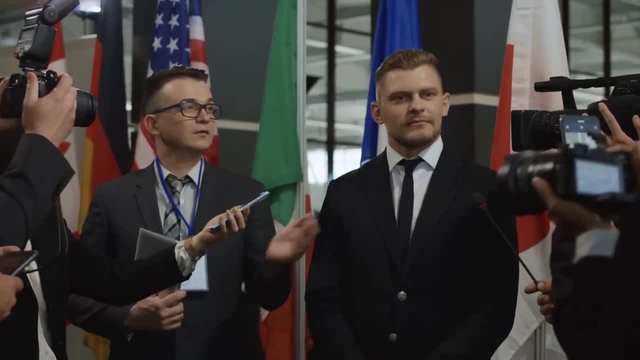 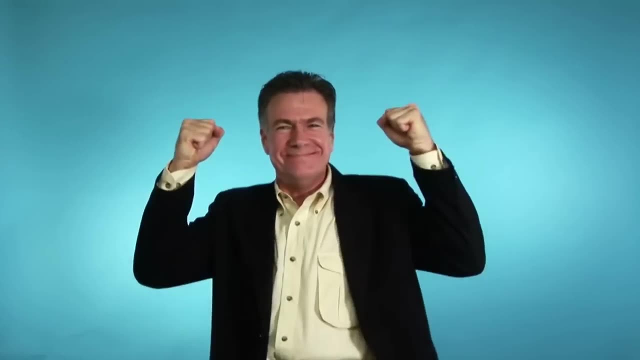 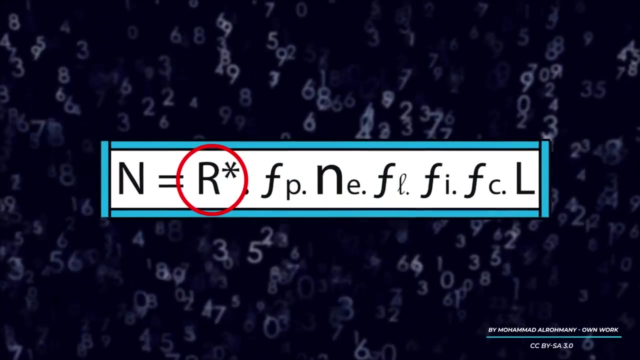 Also, the press releases in particular give the public a false sense that we know the answer or that these arbitrary estimates somehow represent evidence. The real thing is that we just know the first two numbers in the Drake equation: r-star and f-p. 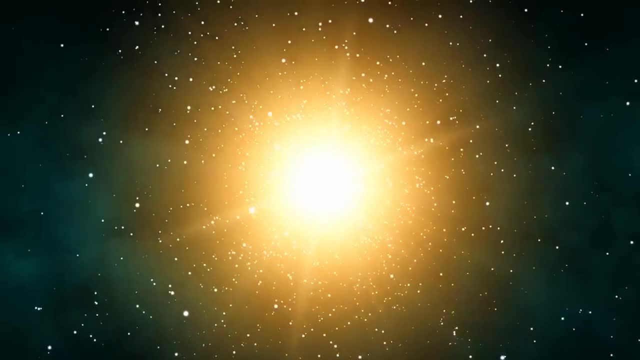 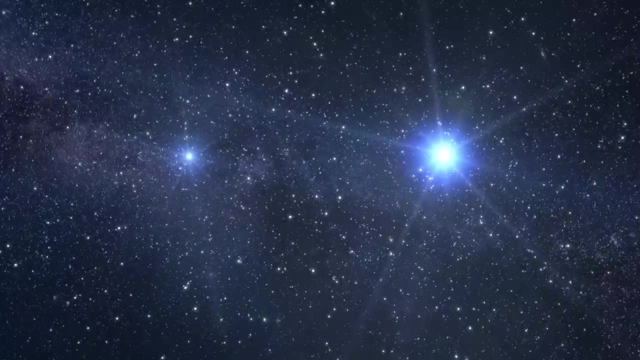 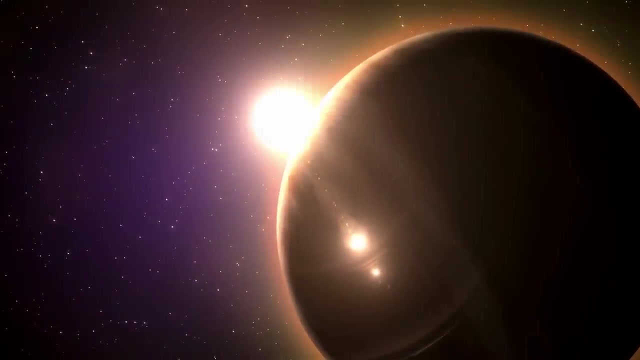 But that's about it. The rate of star formation is something we can absolutely measure and pin down through the detection and study of young stellar objects. We can estimate that the current rate of star formation is about two per year. The fraction of stars with planets is also eminently observable. 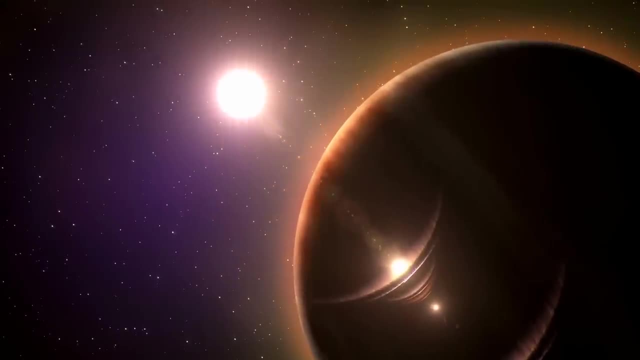 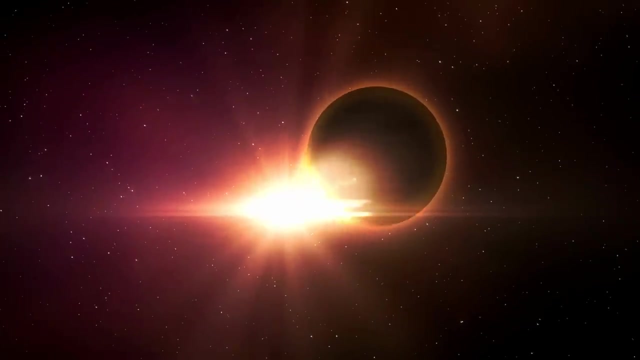 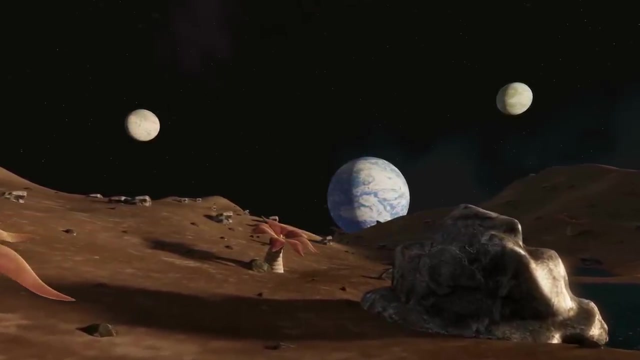 And recent estimates from Kepler and microlensing studies suggest that it's close to one. Planets seem to be a natural byproduct of star formation. The next term is the average number of planets around each star capable of supporting life, And this is where we enter terra incognito. 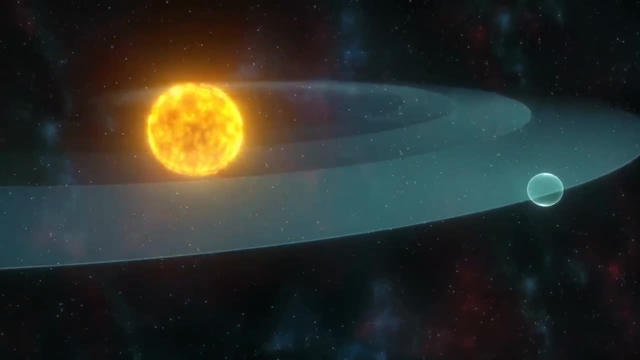 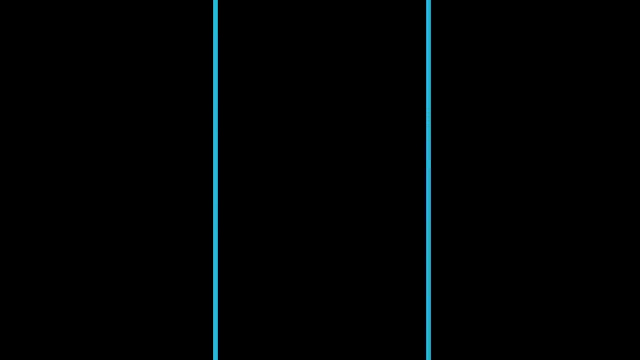 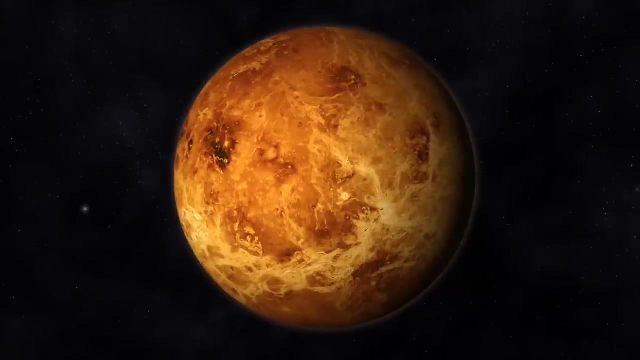 Take, for example, our solar system. There are numerous definitions of the habitable zone that lead to anywhere from one- just the Earth- up to three: Venus, Earth and Mars. But clearly Venus is pretty different from Earth. Yes, maybe it might be possible for it to support life. 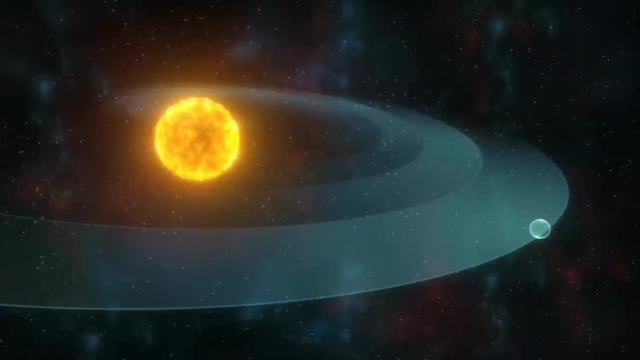 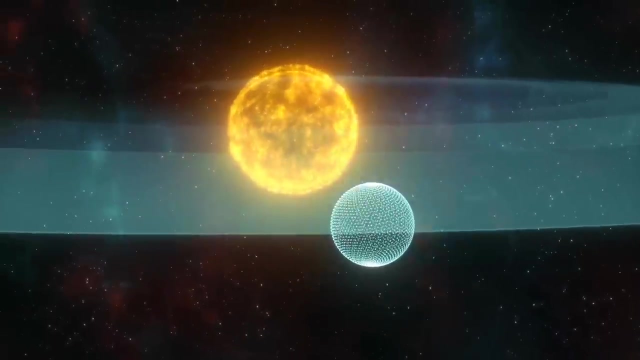 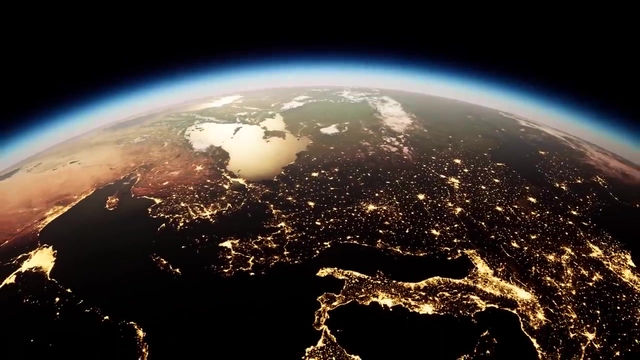 But intelligent life? We don't know. Our surveys can count how many Earth-sized planets are in the habitable zones of their stars. We have no way, with these surveys at least, to distinguish between Venuses and Earths, Or indeed, presumably, other types of planets. 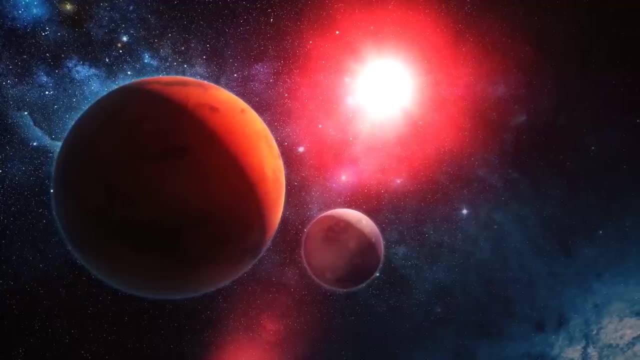 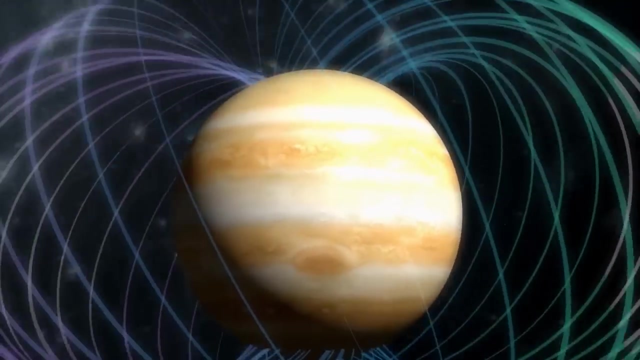 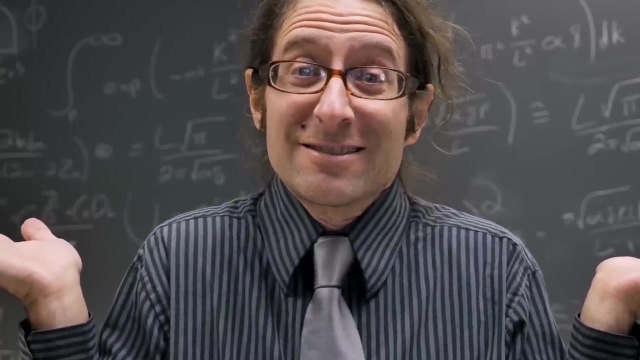 that we've simply never seen before. And this doesn't even touch on other criteria like plate tectonics, obliquity, magnetic fields, etc. So really we don't know this number, but we can actually make progress if we just redefine it. 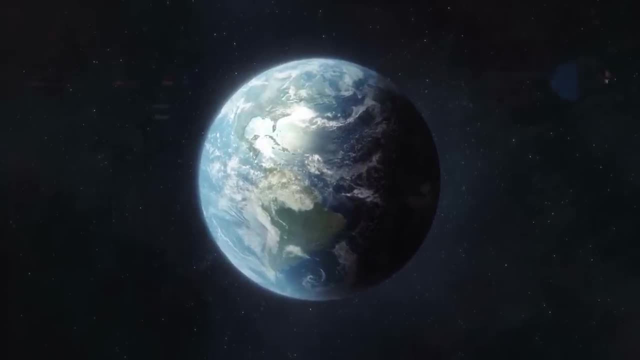 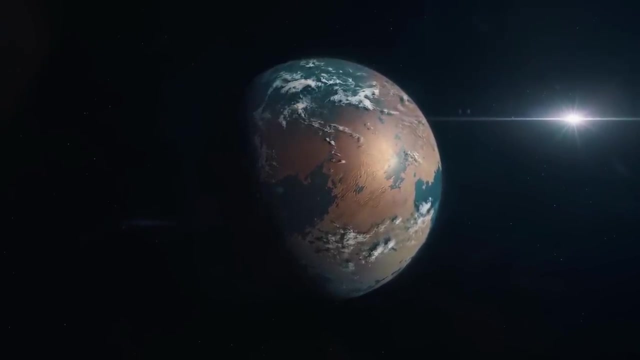 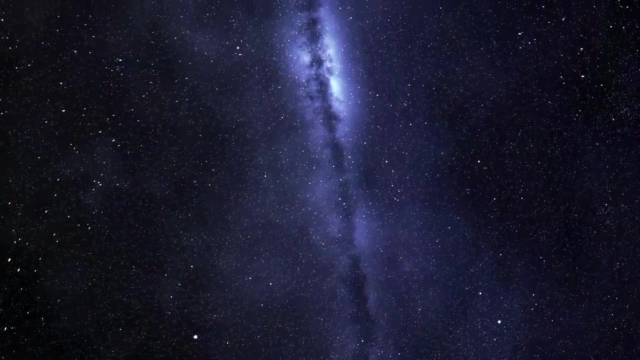 If we consider it to be the number of Earth-sized planets in the temperate zone of their stars, that's tractable. That's a number we can potentially measure. But by casting a larger net like this we would end up making the other term smaller. 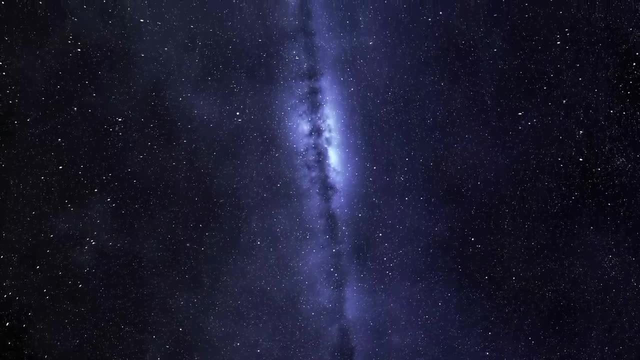 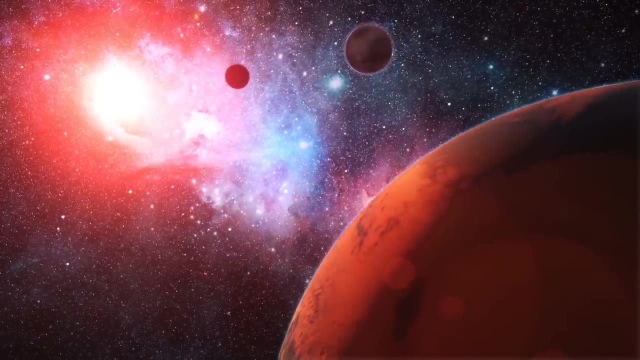 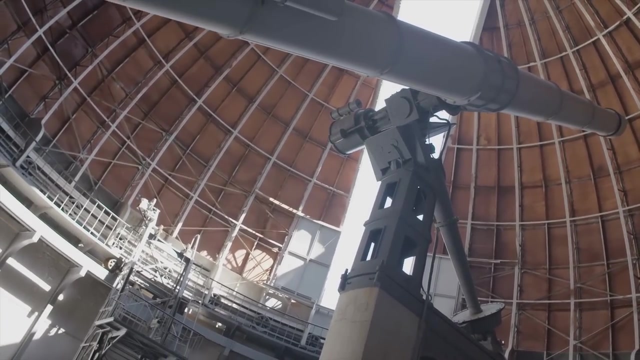 since it's now defined over a wider span of worlds. But at least this makes N an observable quantity. Having said all of that, we actually can't even agree on how many Earth-sized planets are in Earth-like orbits anyway, With modern estimates from the same dataset. 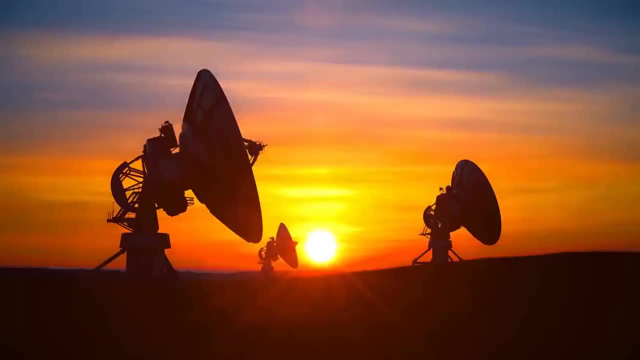 we can see that the number of Earth-sized planets is varying by a factor of a hundred. Nevertheless, in principle, this is a number that we can hope to measure with near-future surveys. Now, as we move on to the subsequent parameters in Drake's equation, 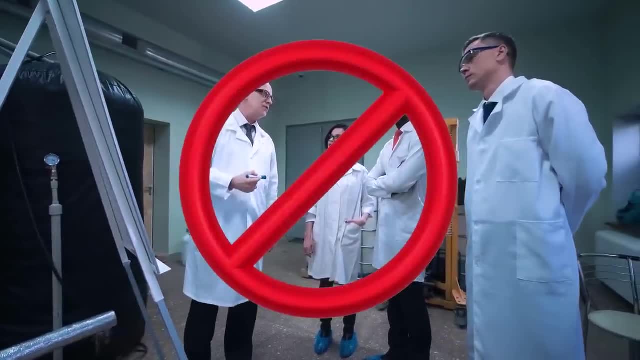 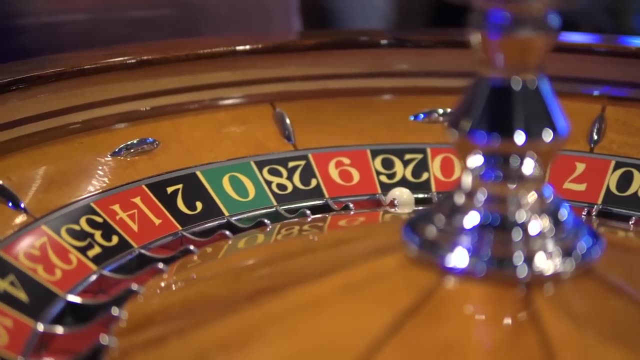 our ignorance only gets worse. The uncertainty here is so extreme it's not even possible to define it in a meaningful sense. So any calculation you see about the Drake equation would suggest all of the terms except for maybe the first two. The perpetual torrent of articles. 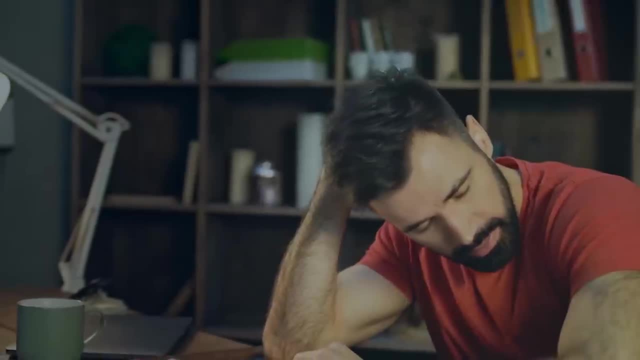 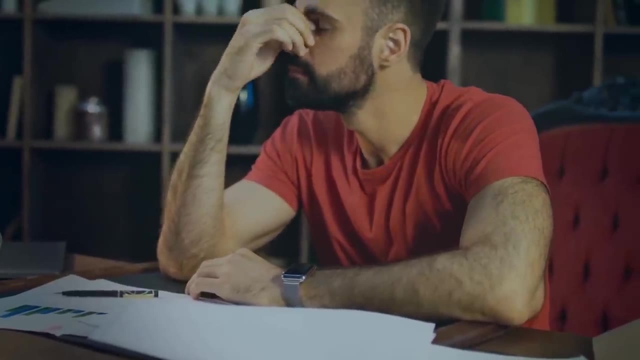 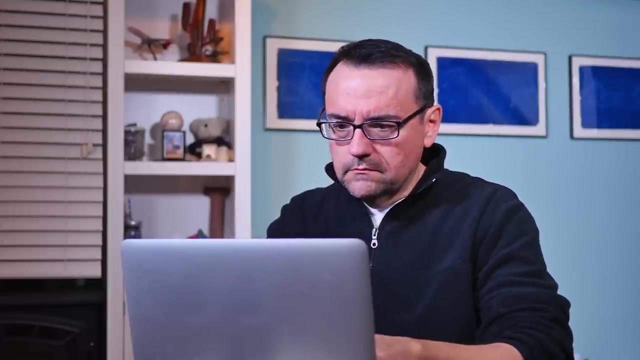 claiming to estimate N in the Drake equation has frustrated and exacerbated many astronomers to the point where now, where they see such articles, many astronomers either ignore them or actively disparage them. The Drake equation has been abused so many times, with the media circus being dragged out. 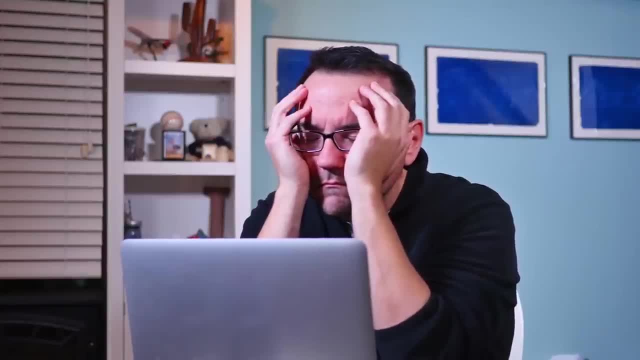 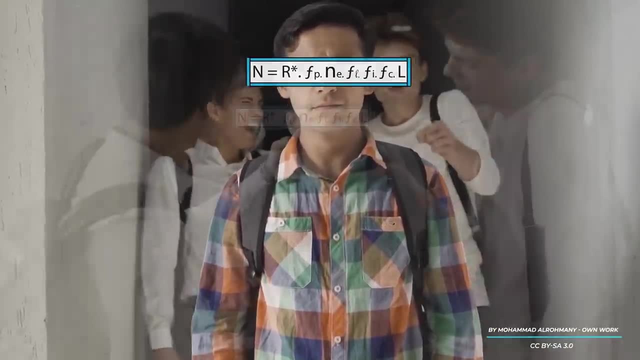 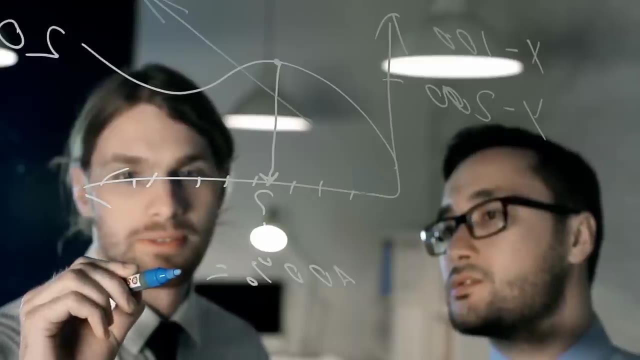 and glammed up for another round of misleading. Nowadays, the Drake equation is now often marked and ridiculed in many academic circles. Many astronomers not only don't trust the Drake equation, they really hate it. But here's the thing. Yes, there are undoubtedly flaws with the Drake equation. 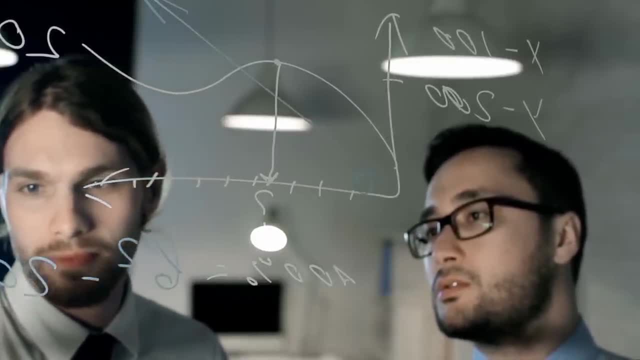 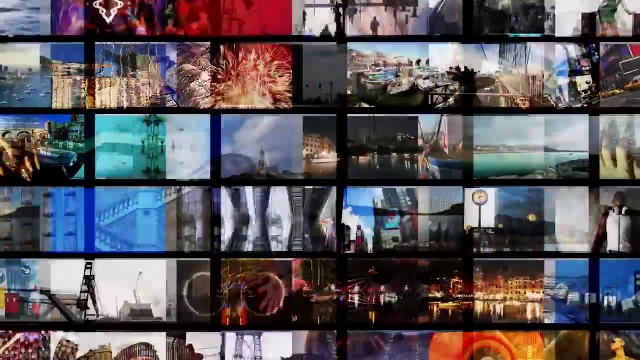 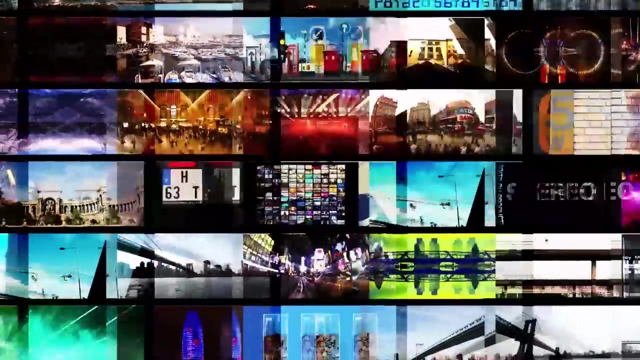 but much of the bad reputation that it offers is a product of its past abuses and not its original formulation. All of this is undoubtedly largely fair and arguably largely fueled by the media circus that tends to come along for the ride In the last part of the video. 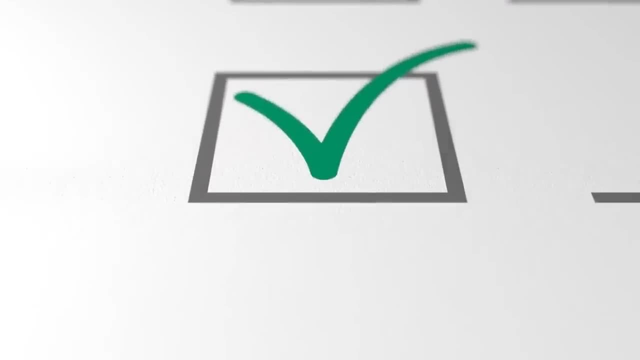 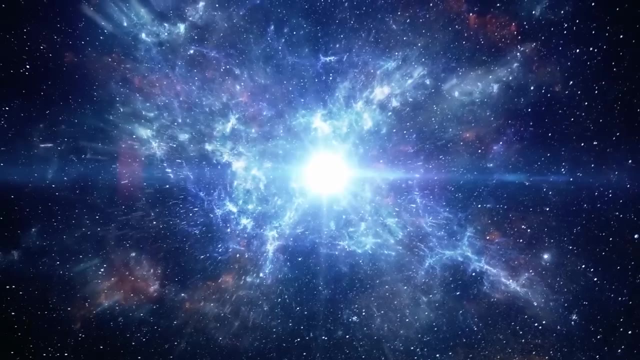 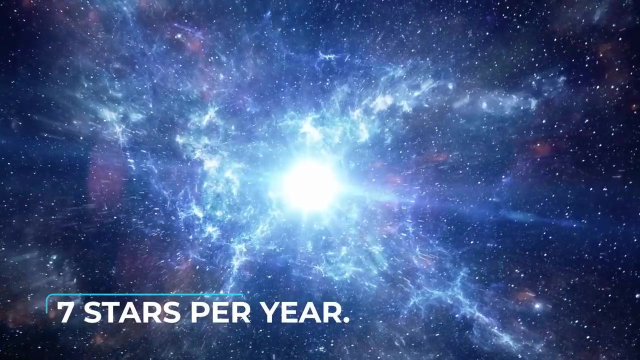 we try to provide a list of the most reliable estimates of the parameters that appear in the Drake equation: Our star, the star formation rate in the Milky Way. The most recent calculations by NASA and ESA indicate that the current star formation rate in our galaxy is 7 stars per year. 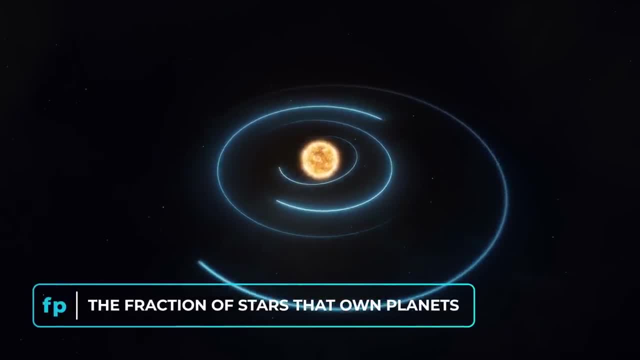 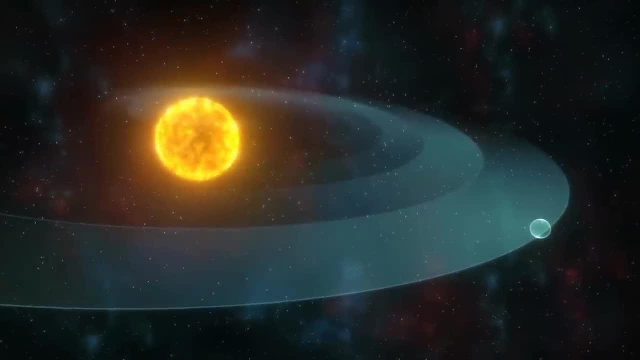 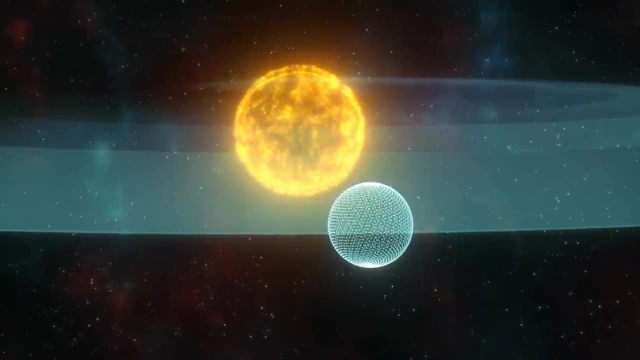 Fp, the fraction of such stars that own planets. Recent research on exoplanets has shown that 40% of sun-like stars have planets, and the real fraction could be much greater, as only considerably more massive planets than Earth can be detected with current technology. 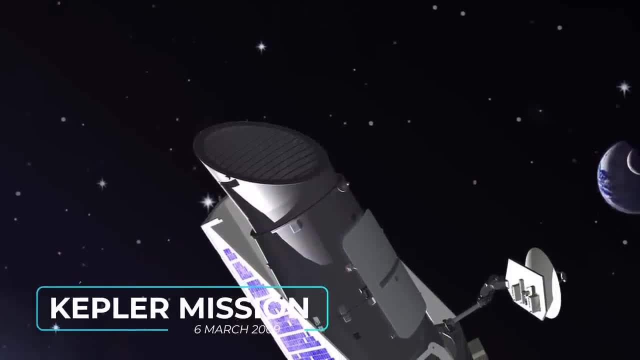 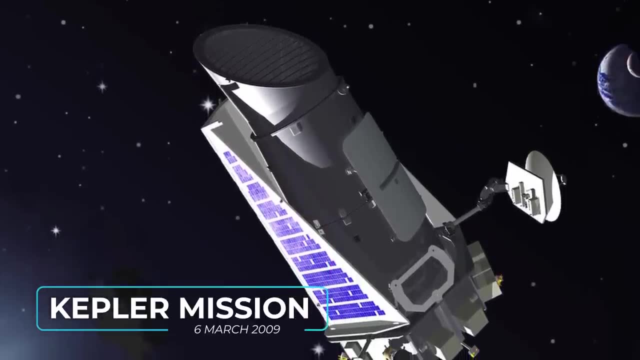 The Kepler mission of NASA started on March 6, 2009.. It should provide an estimate more accurate in the number of planets per star located in a habitable zone. In fact, it can count on instruments much more sensitive than in the past. 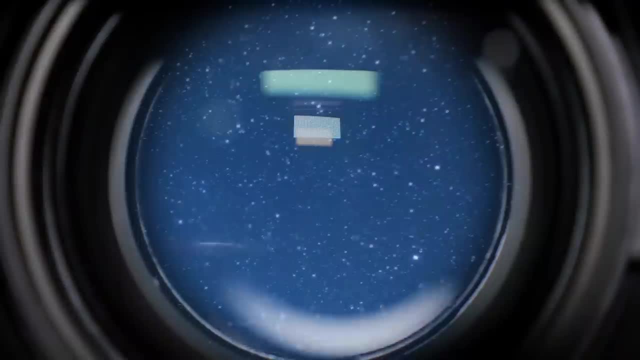 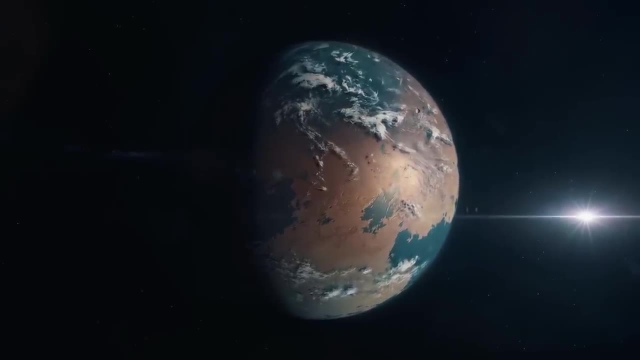 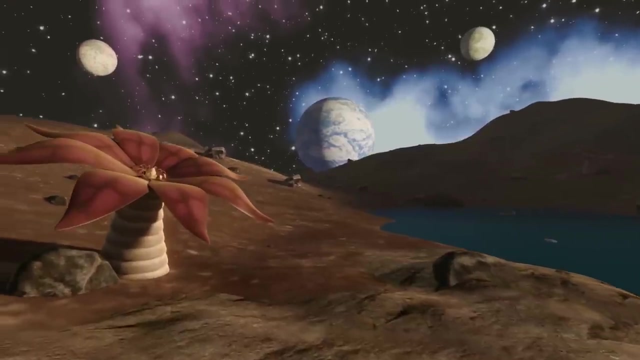 capable of detecting planets as large as the Earth with orbital periods of up to one year. Even if we know the number of planets that are in the habitable zone, however, determining how many of them have the right combination of factors can be difficult. 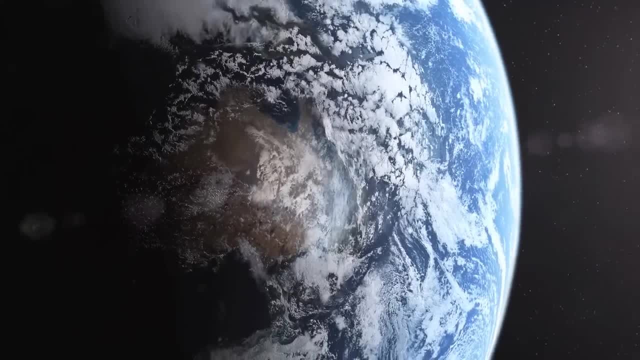 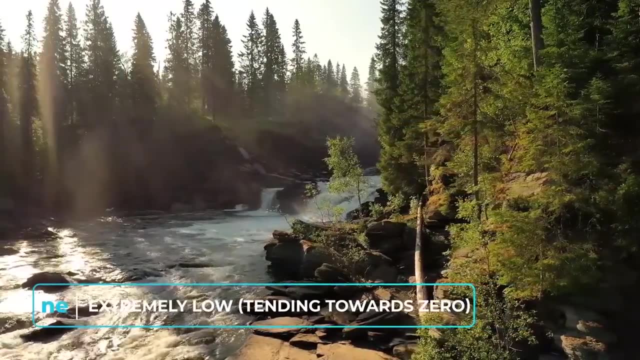 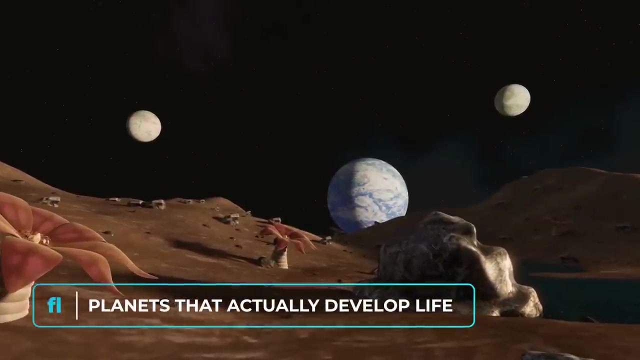 Furthermore, if the hypothesis of the rarity of the Earth is valid, the set of characteristics verified on Earth may not be common at all And the number Ne could be extremely low, tending towards zero Fl, the fraction of them that actually develop life. 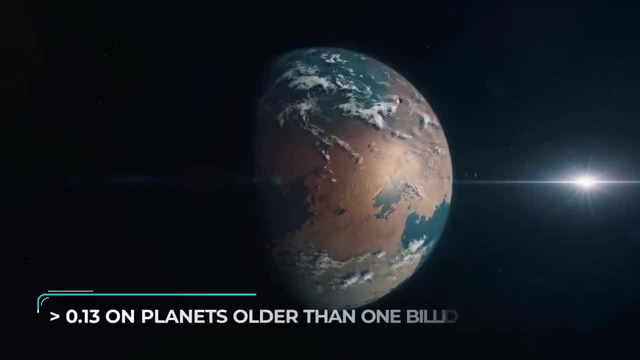 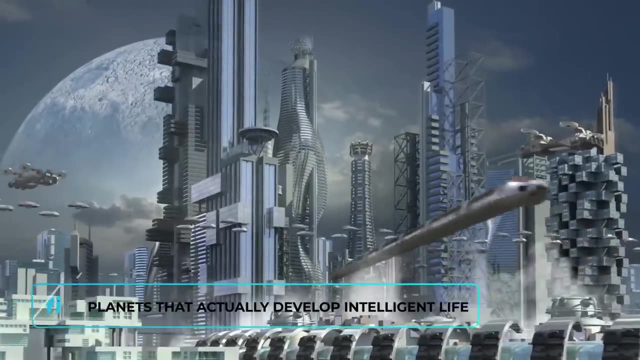 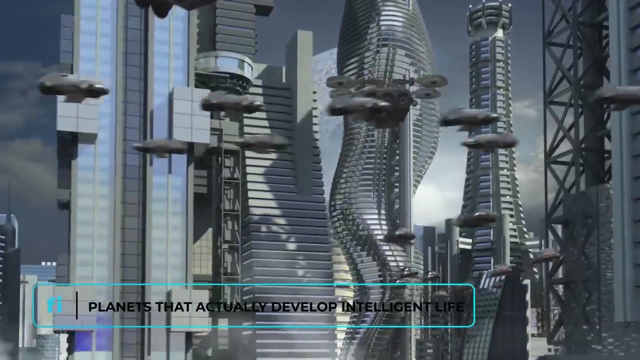 We don't know very much about it. It must be greater than 0.13 on planets older than one billion years Fi, the fraction of them that actually develop intelligent life. This value remains particularly controversial. Those who speak out in favor of a low value. 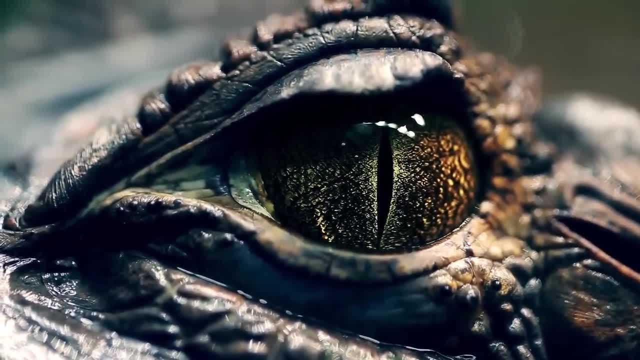 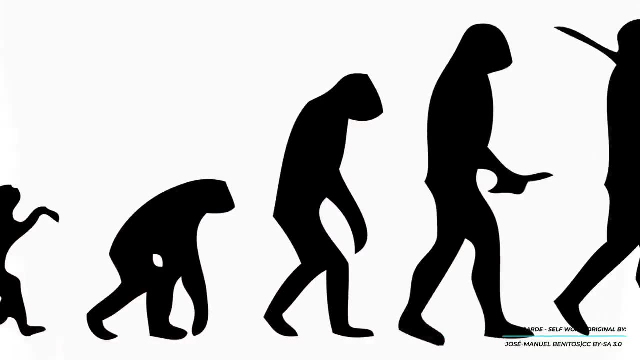 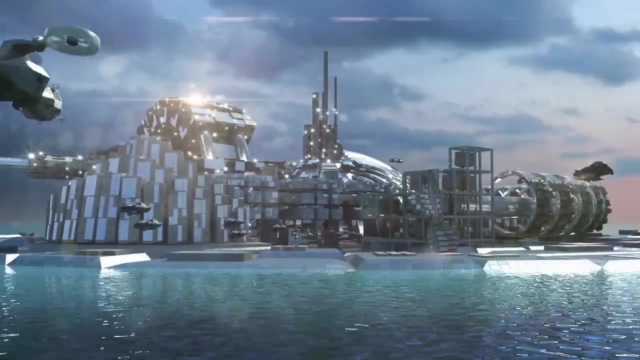 point out that, of the billions of species that have existed on Earth, only one has become intelligent. Those who are in favor of higher values emphasize instead that the complexity of living beings tends to increase along the course of evolution and conclude that the appearance of intelligent life 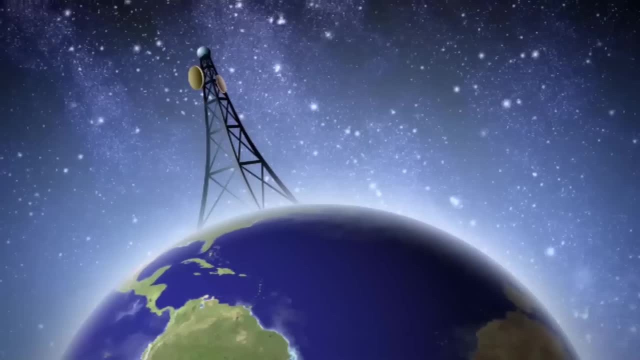 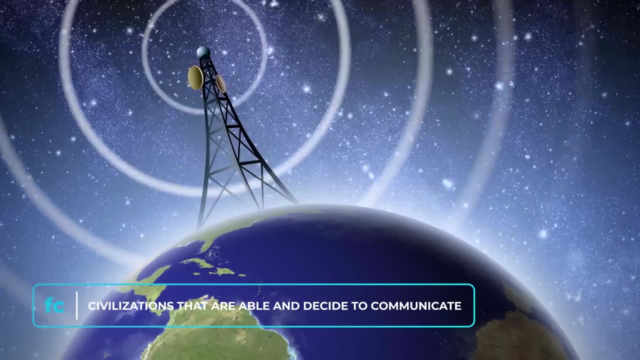 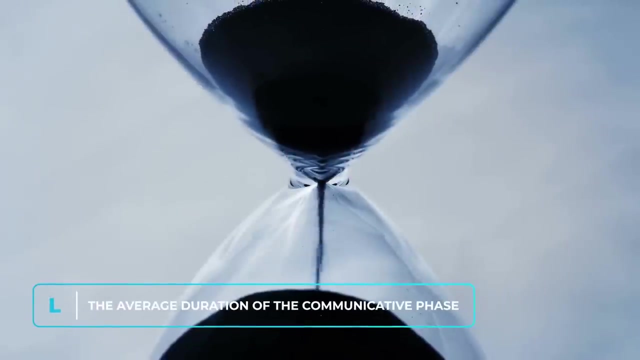 sooner or later, is almost inevitable. Fc, the fraction of them that is able and decides to communicate. Although much speculation has been made, no concrete data is available on this parameter L: the average duration of the communicative phase of each of these civilizations. 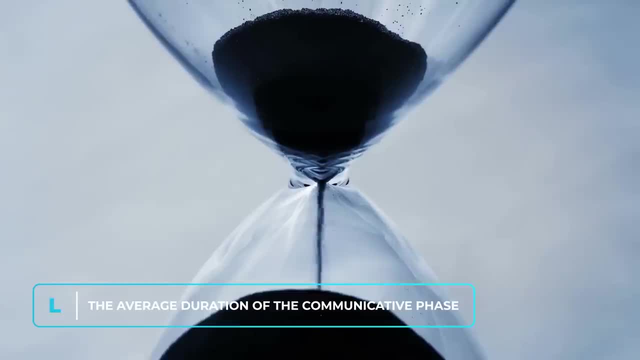 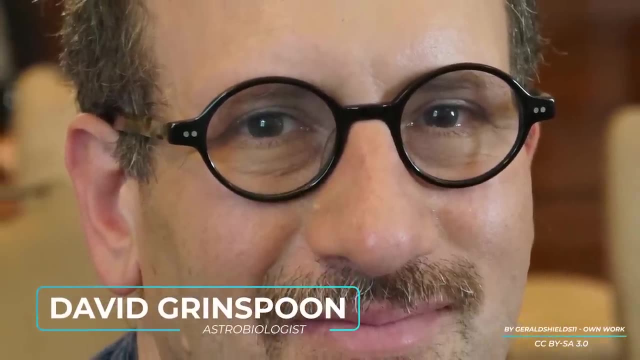 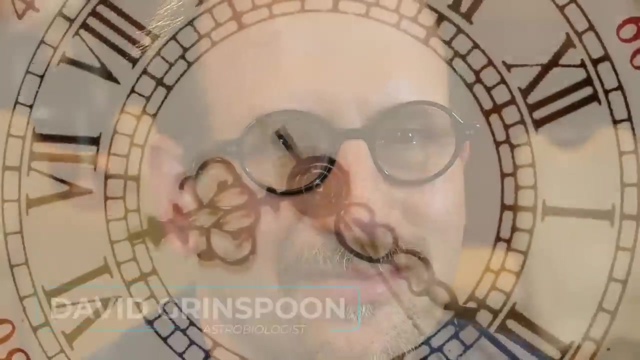 Some values were proposed: 420 years, 304 years. Others, such as astrobiologist David Grinspoon, have suggested that once a civilization had developed, it could overcome all threats posed to its survival And then survive over an indefinite period. 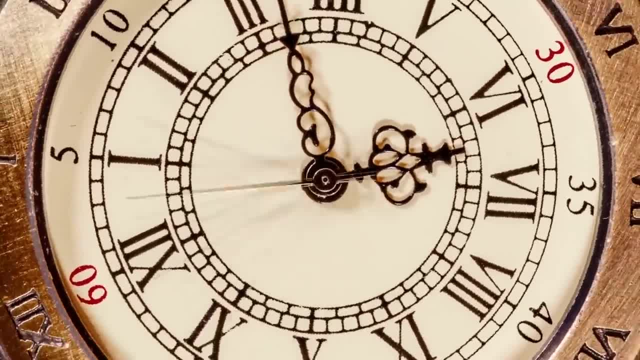 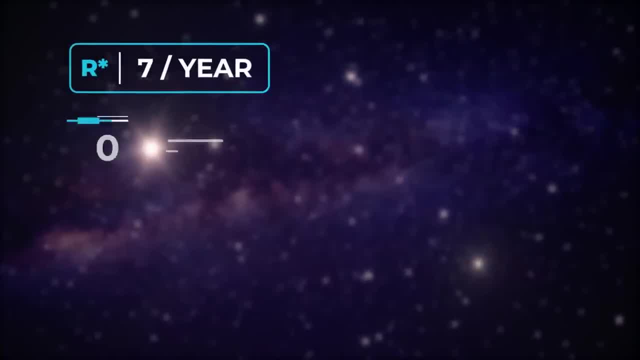 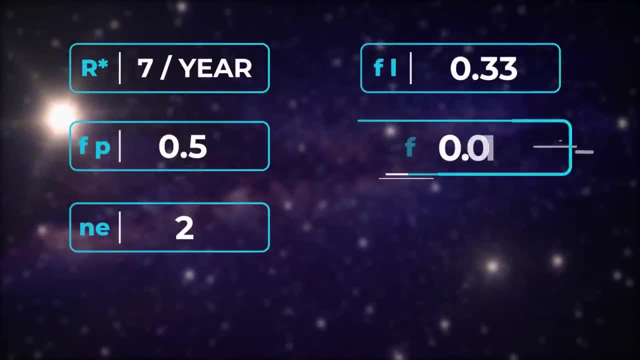 bringing L to the order of billions of years values based on the quoted estimates. R star equals 7 per year. Fp equals 0.5.. Ne equals 2.. Fl equals 0.33.. Fi equals 0.01.. 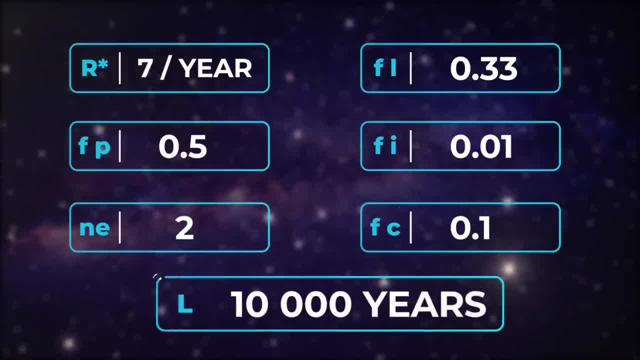 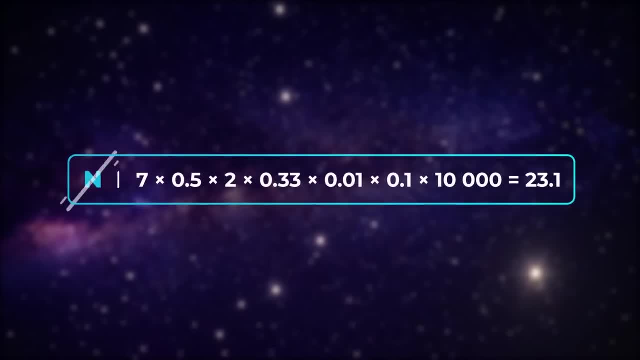 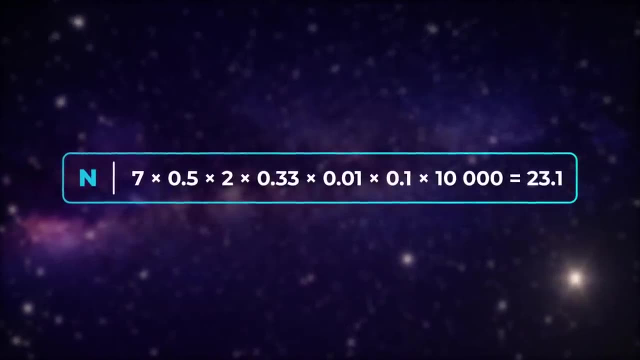 Fc equals 0.1.. L equals 10,000 years. Gives a result: of N equals 7 times 0.5 times 2 times 0.33 times 0.01 times 0.1 times 10,000. 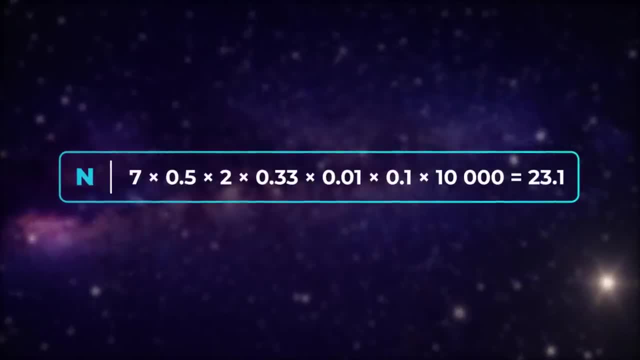 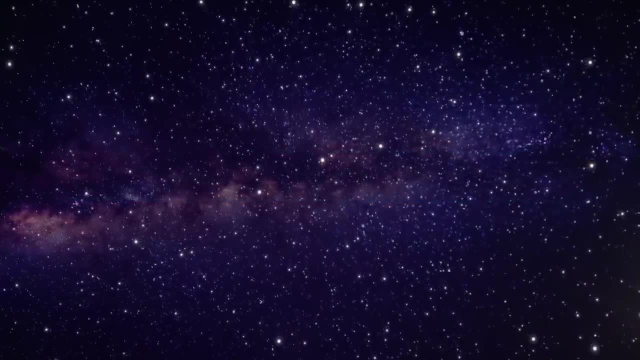 equals 23.1.. Existing extraterrestrial civilizations capable of communicating in our galaxy. Drop a line below, so we know if this is the result you expected. 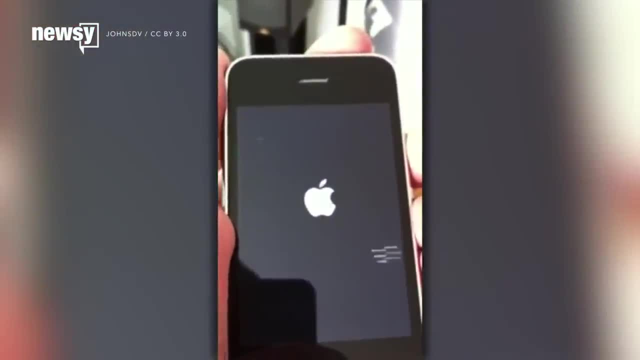 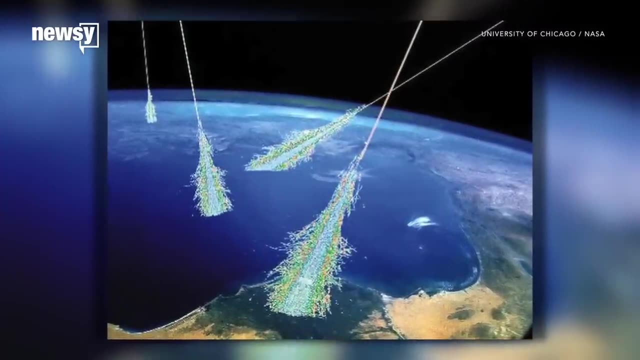 Knock on wood that your phone never crashes, But if it does, cosmic radiation could be to blame. Researchers at Vanderbilt say electrically charged particles raining from the sky can be a surprisingly big problem for personal devices, And the problem is growing. The cosmic 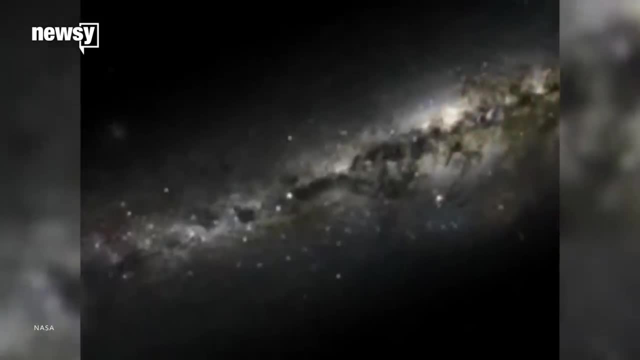 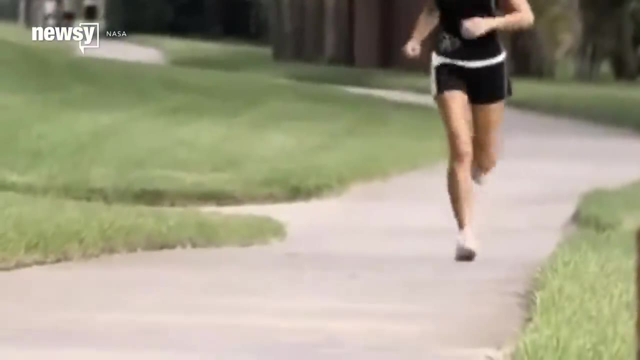 rays we're talking about don't come from the sun, but from outside our solar system. These rays hit Earth's atmosphere, creating subatomic particles. Millions of these hit your body every second without any known side effects. But electronics are a different story, Because 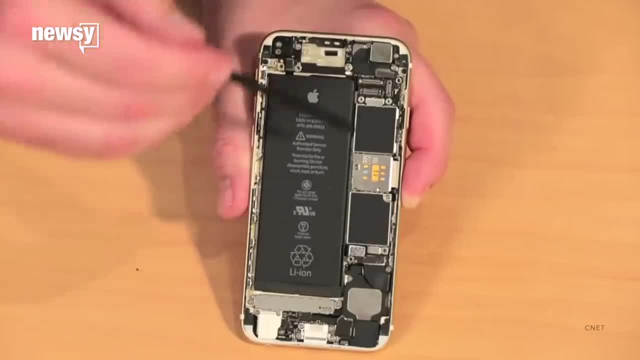 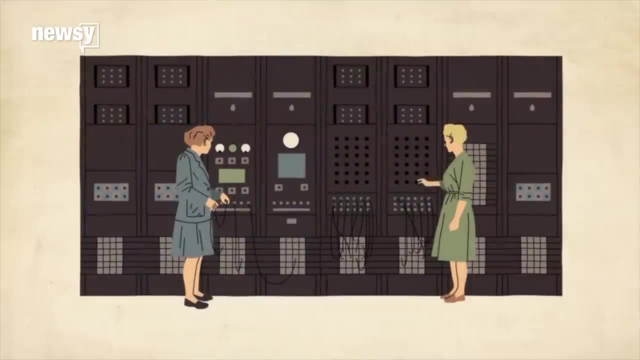 some cosmic particles have a charge. they can mess with the device's circuitry and stored data. Fixing this kind of problem for your phone may require a hard reset, which could be a personal nightmare. The fact that transistors and computers keep getting smaller could raise 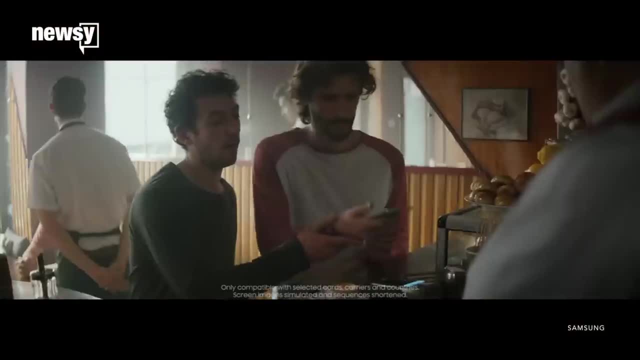 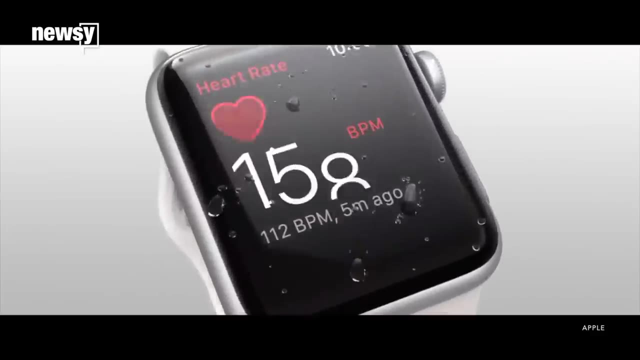 the risk of cosmic rays interfering with circuitry. The researchers also note that particles have more potential targets. since there are more and more computers in our society, We're relying on computers more too. While cosmic rays may seem bad for your personal devices, they've 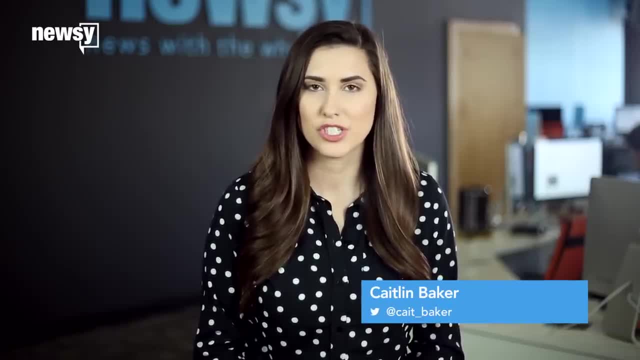 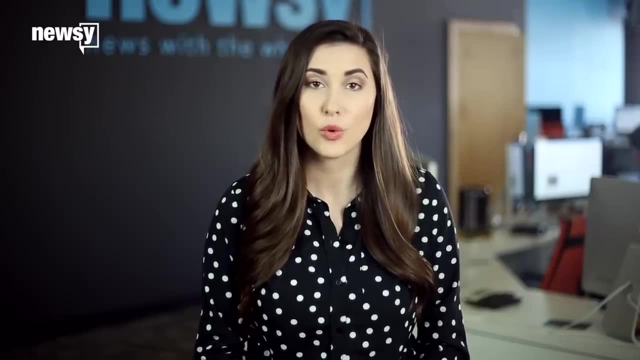 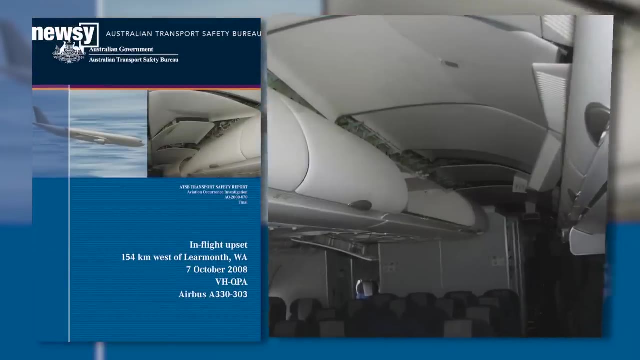 actually caused more serious problems in the past. Researchers suspect the rays changed a single binary digit in a Belgian voting machine in 2003,, giving a local candidate 4,000 extra votes, And in 2008,. rays may have caused a plane's autopilot system to malfunction. The plane dropped 690 feet in less than 30 seconds.